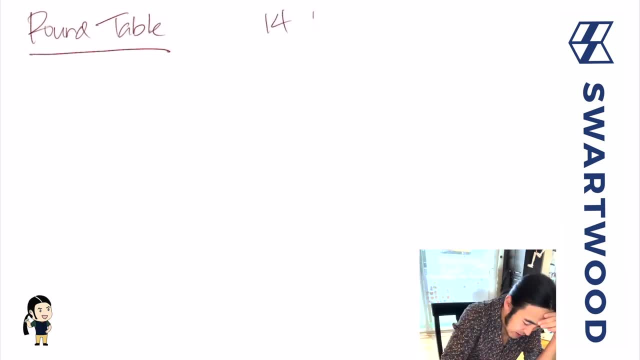 So my take on this is: first, what is the problem? The problem is you've got a roundtable and they always sit the same way around the roundtable, so they kind of have assigned seats okay, And I like to pick three for a quest. 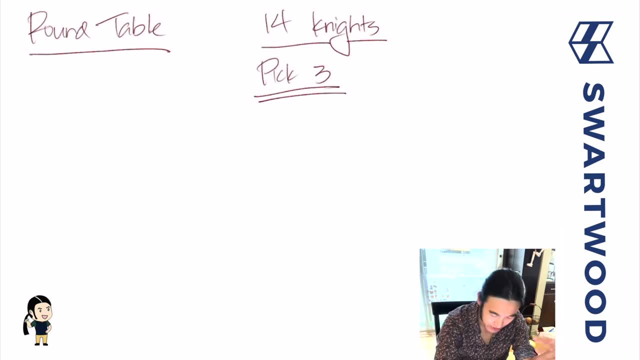 Okay, for those of you that like that sort of thing, this is kind of an homage to Sir Thomas Mallory. the 14 knights: I think Mallory estimates something like 140 knights at the roundtable, so we're going to go down to 14, okay, But you want to pick three knights and there's a stipulation. 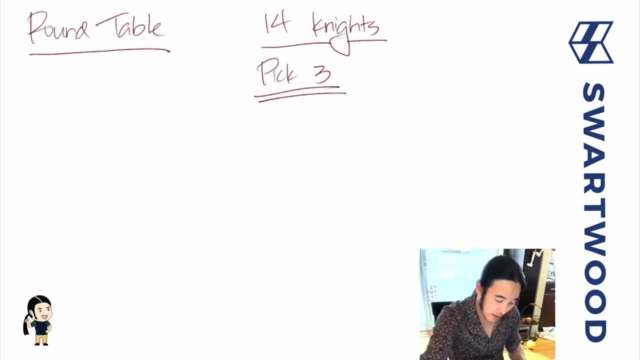 So the three knights you pick cannot be seated next to each other. okay, So no adjacent knights, or at least no adjacent knights that are picked. Okay, all right. so how do we do this? So I think one of the quickest ways to do this is first pick a distinguished knight, because it'll help. 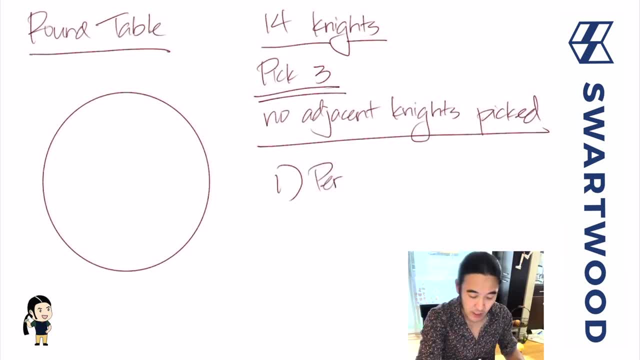 orient us okay. So remember they always sit the same way at the roundtable. So what we're going to do is we're going to pick a knight- let's say we pick Percival, okay, And wherever Percival is, because he's always assigned at a certain seat. 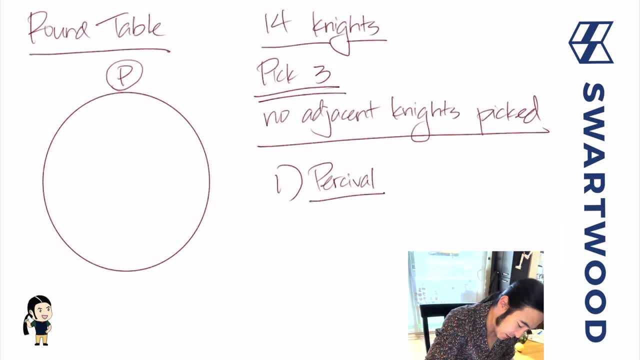 we're going to take that. take him, move him around so he's at the head of the table. That'll just make life easy for us. okay, And now? how many other knights do you have to pick? We have to pick two more, so they're out there somewhere. okay, All right, those will be the 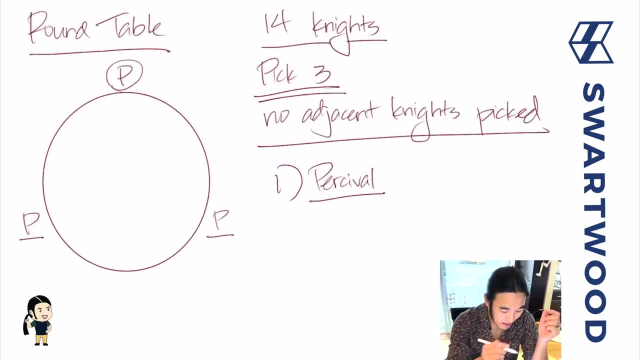 other picked knights. So how do you know which knights they are? Well, if you knew the number of knights, let's say, between Percival and the first picked knight, and you knew the number of knights between Percival and the second picked knight, well definitely you would also know the number of knights between the two picked. 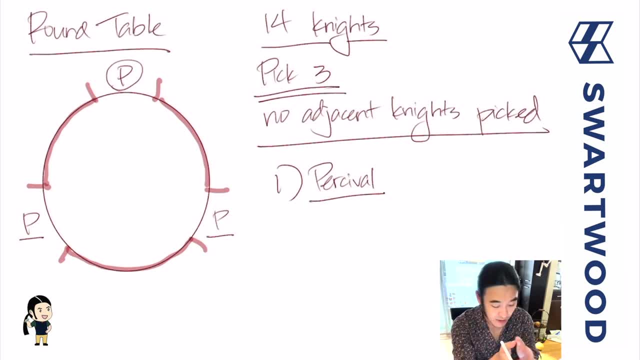 knights like this right. So if you knew this, then you would definitely know who's seated where. okay, So our goal is going to be this: Let's first look at all the knights out there. They're 14.. We have placed down Percival and his two friends, so that's going to be three placed down. Now we 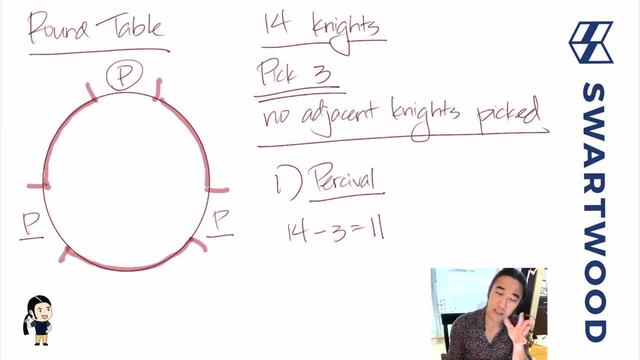 have 11.. Now the stipulation is that none of the picked knights can be adjacent, So the guarantee that we're going to place at least one knight between each of the picked knights. Okay, so that's going to use up three more. Then we have eight. All right, but the other eight knights 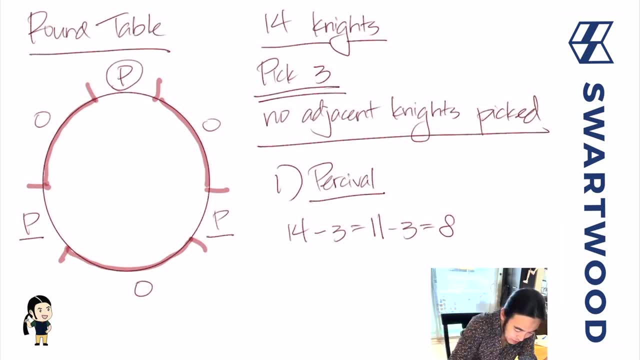 they can go wherever And all that really matters. like if I were to place, say, two knights here right or place two knights there, it doesn't really change anything because that's the same number of people right between Percival and the knight on the right. So all that really matters is: 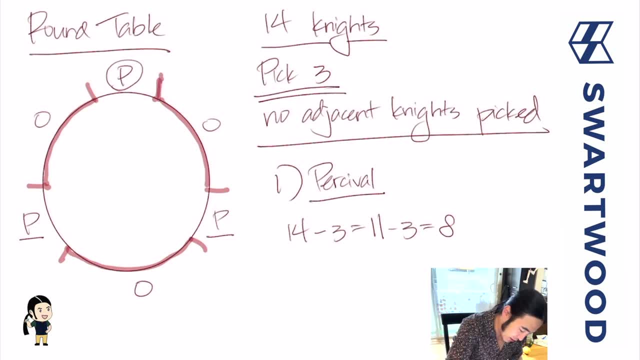 we're looking at these buckets again. So bucket number one, it should be a different color, huh, Bucket number one. bucket number two: okay, and bucket number three: All right. so all that matters is the number of the remaining knights that we place in each of those buckets. So it's equivalent to saying, well, we've got. 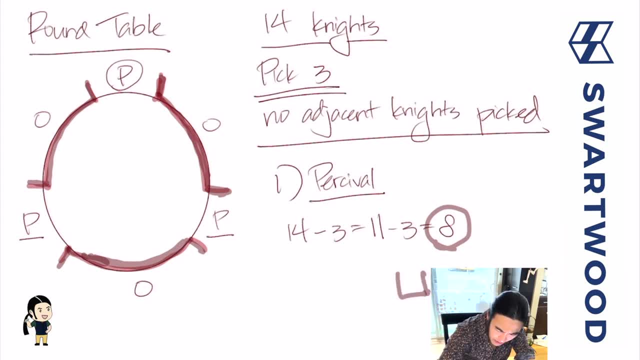 three buckets. Again, I'll put links in there if you want to reference the old videos, because I'm going to assume you're comfortable with the old videos. So if I have three buckets and I need to place eight knights inside of them, right? So I'm going to put three buckets in there and I'm going to 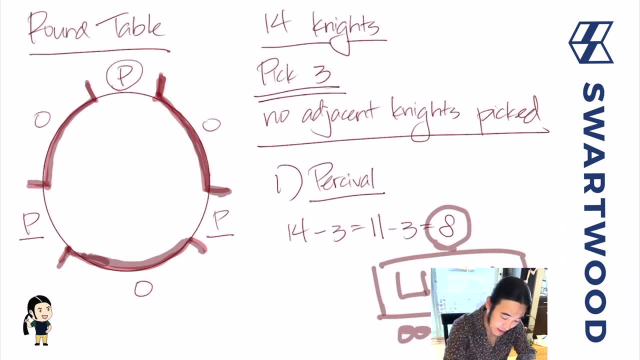 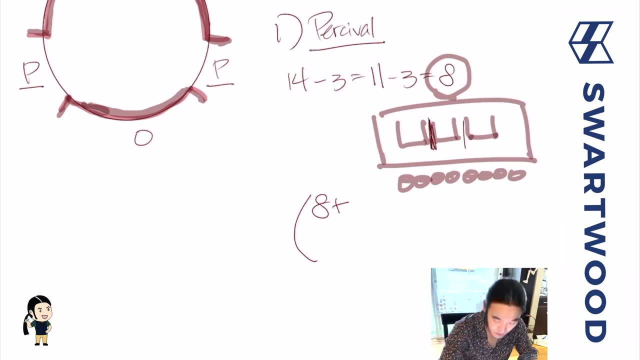 So eight like this? How many ways can that be done? Well, we've talked about this before. You take your eight right and you need three buckets, But three buckets are defined by two dividers, So it's really going to be three minus one for those two dividers. Choose where the dividers go, and this: 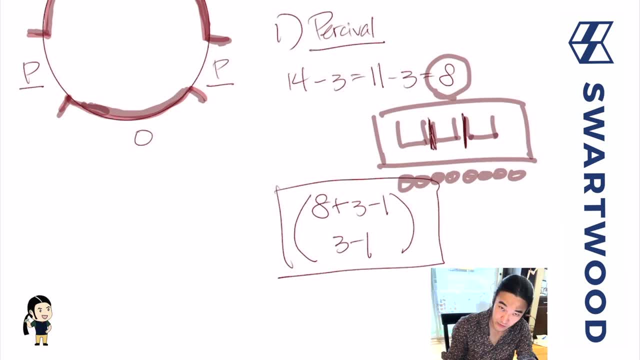 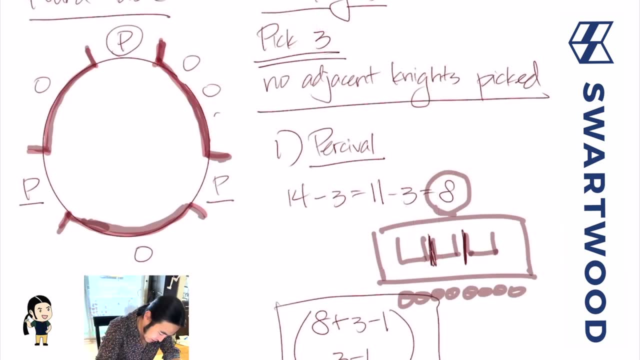 would pretty much be our answer- Not quite the answer to this problem, but pretty close, okay. So now, what have we done? We've set everything up. We know exactly where the knights sit. Let's make it hypothetical. Let's say we place the eight this way: One, two, three. 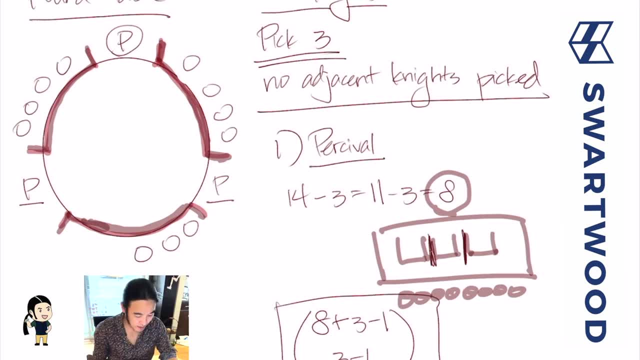 four, five, six, seven, eight, okay, Something like that. So that would place down pretty much all the knights. They sit in a certain order. So if we know where Percival is and we know how many are to the right and how many to the left of him before you hit the picked knights, right then for 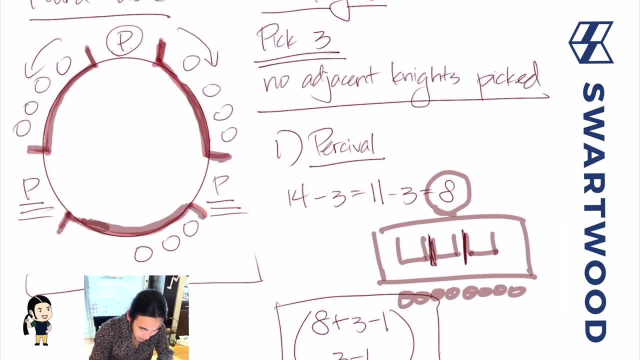 sure we know what this range looks like. okay, There's only one slight problem with this, and that is we made Percival distinguished, right? We said, okay, we started the counting, assuming that you know Percival is a special knight we're going to pick, But it doesn't have to be Percival In. 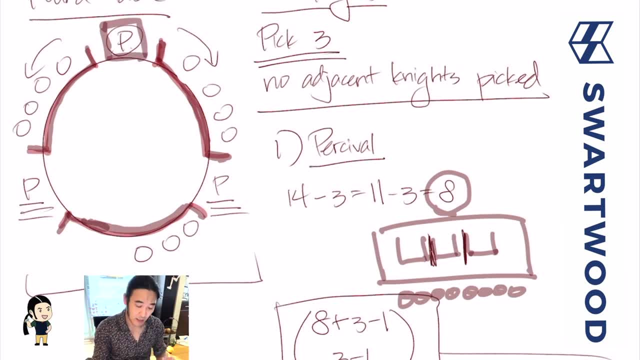 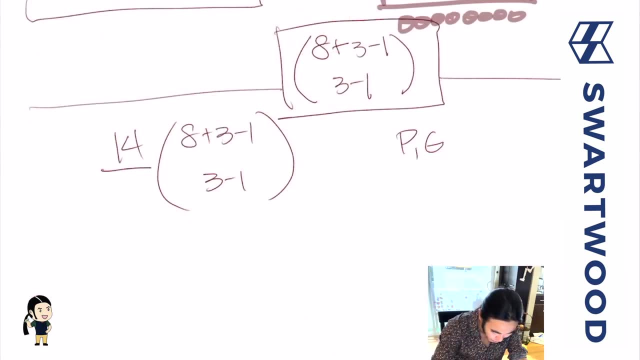 fact, he doesn't even have to be picked. It could have been any of the 14 knights. So to take care of that, we're going to take this number and multiply by 14, which is almost right again, But there's a slight problem. So let's say we 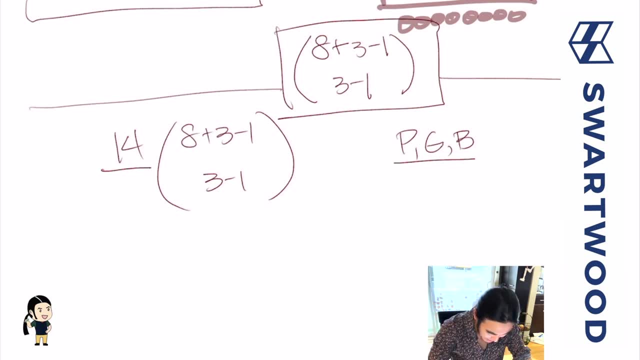 picked for our three knights: Percival- I don't know- Galahad and Bors. So Percival, Galahad and Bors, We picked these three knights. okay, And one way in the way we've counted right. 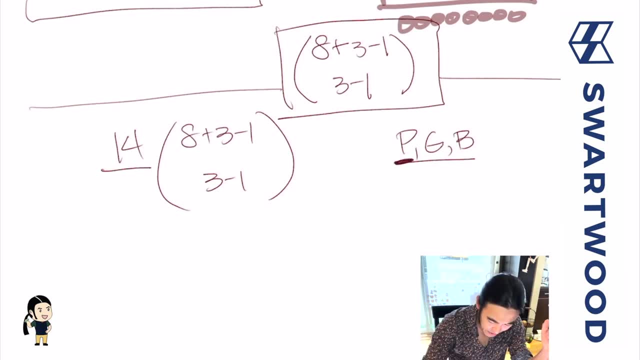 we kind of picked that lead knight. So in one version of this I picked Percival as the lead knight and then the other picked knights might be Galahad and Bors. But we also, when we multiply by 14, we looked at the possibility where we had Percival. 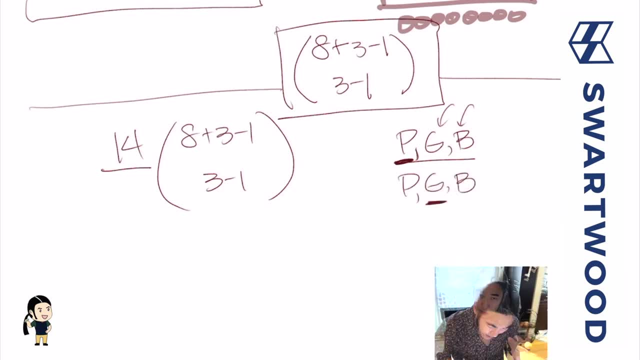 Galahad and Bors. And Galahad was the one we picked, And there's also a version where we get the same group, but Bors was the one that we picked. We made the distinguished leader, okay. So because of that, we've overcounted, right? So for this group of three, we've overcounted. 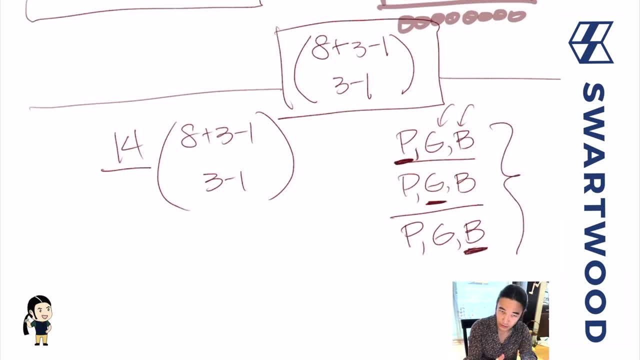 three times because we could use any one of the three to sort of be the leader. So to fix that, every time we're overcounting three times, we divide by three. So this is actually the solution. Okay, So it's a pretty fast solution to a classic problem. but we're going to generalize and do an 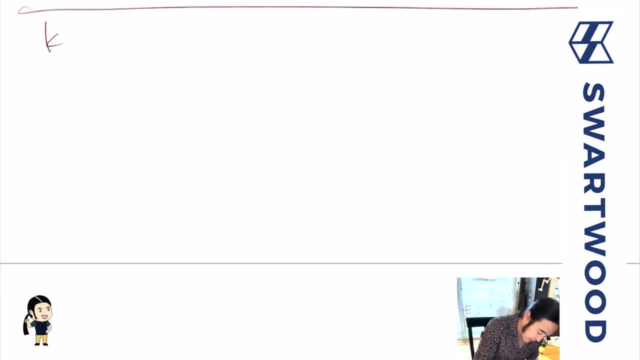 even harder version. So now we're going to have k knights, We're going to pick p of them and the same rules apply. So there has to be at least one knight between each of the picked knights. okay, Same strategy. We're going to pick Percival- okay, at this table. 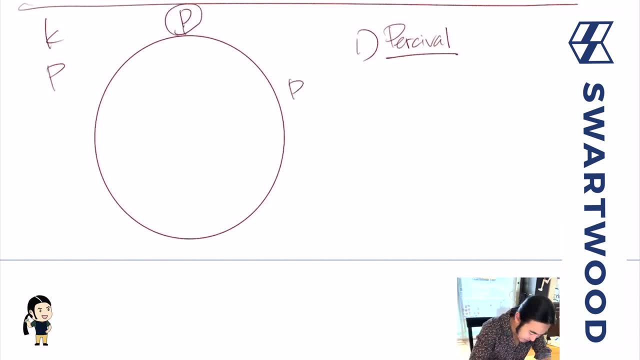 Place Percival down. and now I'm just going to randomly draw some other number of knights. It could be any number, It doesn't have to be you know four of the knights, but I just want to make my point. Okay, So here's our logic. again, We have k knights, We place down Percival and the remaining knights. 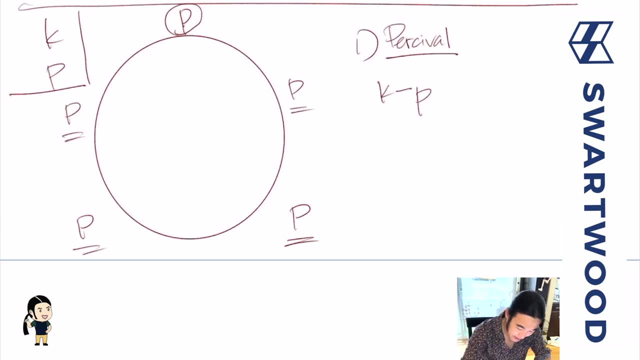 right that we're going to pick. So there's p of them. So we have k minus p knights left, k minus p knights left, Okay, All right. However, we need to make sure there's at least one knight between each of these. So if you have, for example, five guys here, you can see the number of spaces between. 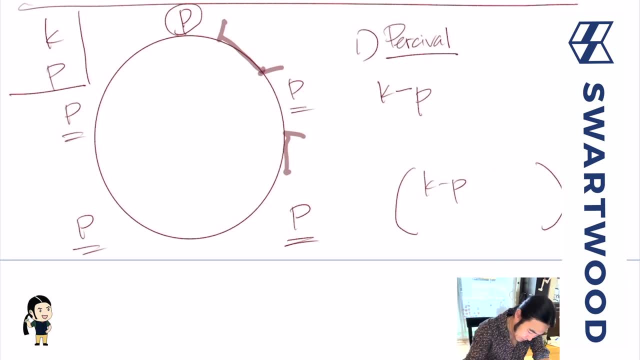 them. the gaps between them is one oops, two, three, four and five. And likewise, if we had p knights in general, like we're doing now, we'd have p spaces between them, So we'd have to place down one, two, three, four, five. 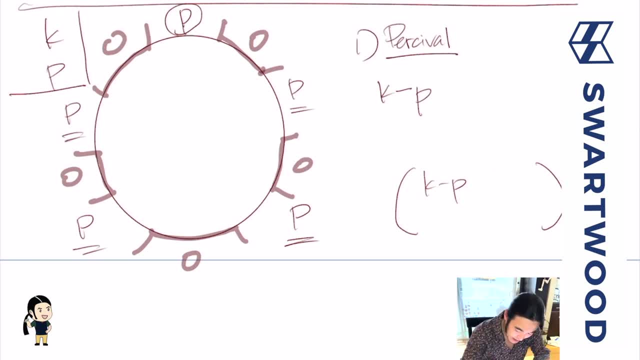 or in general, p. okay, So we need to place down p more knights. So now we have k minus p minus p. knights are left, but we need to place these guys in these buckets, right? So, again, if we knew exactly how many nights were between Percival and this guy, right there, right. 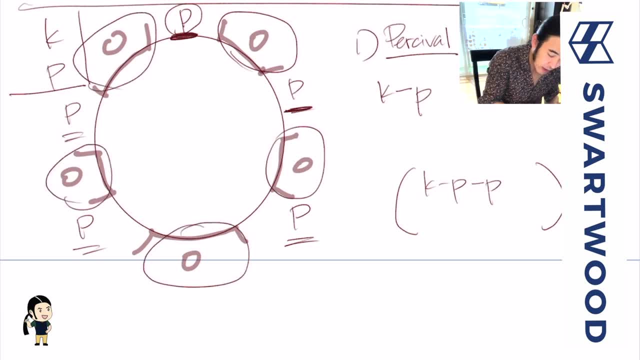 so we knew how many were here, here, here, here and here. we would know exactly what that arrangement looked like. and again, how many gaps we have. here we have five, or in general we'd have P. so if I have P buckets and you place this many nights, 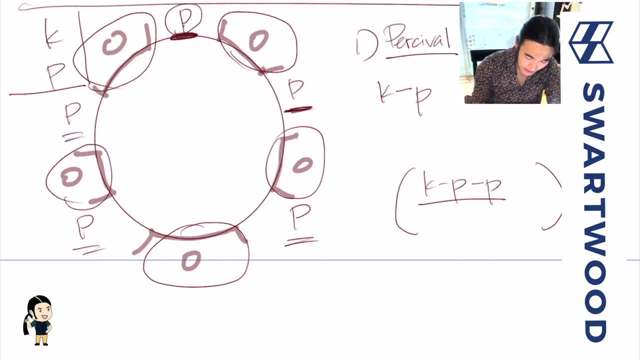 inside those P buckets. right, then I need those nights. plus, I need P minus 1 P minus 1 dividers, okay. so once we have everything set up, if you choose or the P minus 1 dividers go, then we know exactly what everything looks like, okay. 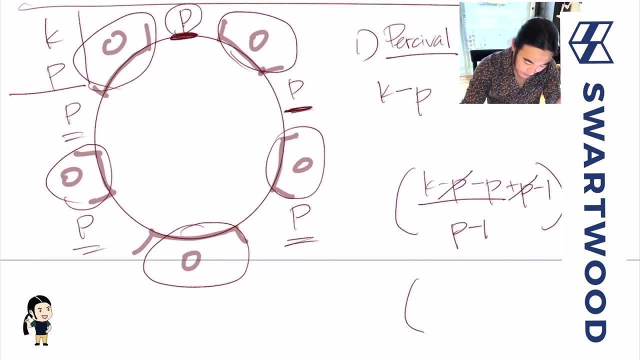 and in this case negative P and positive E cancel out. so this formula looks really pretty. it's K minus P minus 1. choose P minus 1 again. we have the same problem as before. why Percival? why not any of the other remaining nights? so multiply by K, but for every committee of P nights that we picked, we count them. 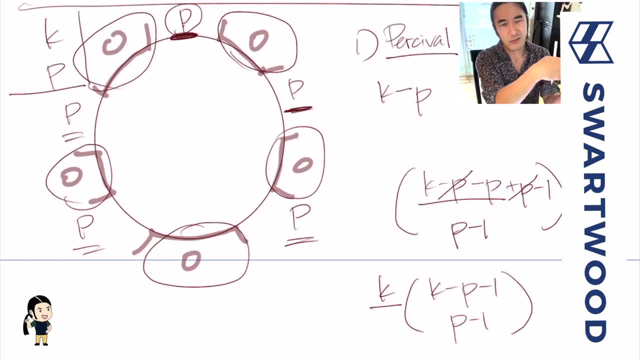 multiple times. right, because we're distinguishing a leader. but it doesn't really matter. when you get that group of nights there is no leader in the group, we just pick them for the quest. so the way we've counted, we said one of them was a leader. but in all those 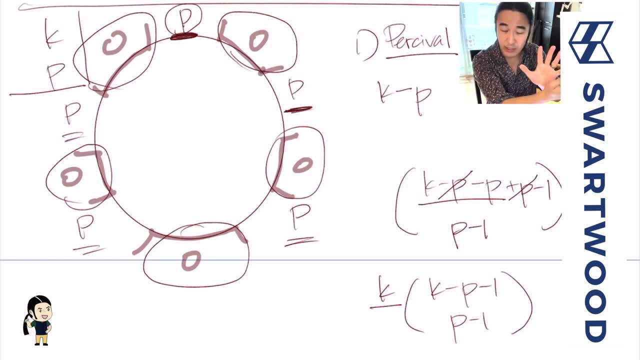 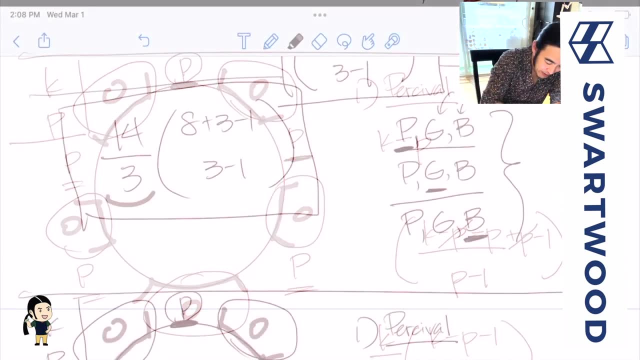 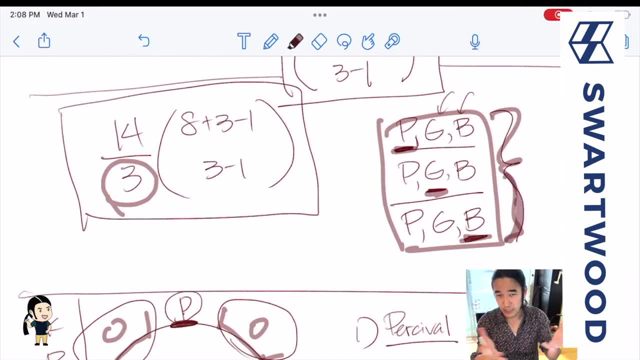 three different leaders for the basically the same group. we made up this whole leader idea to help us count when you get the group of P G B, this is one group, right? all right, so we go back here and this looks like the right answer. okay, does it apply? let's go back to the 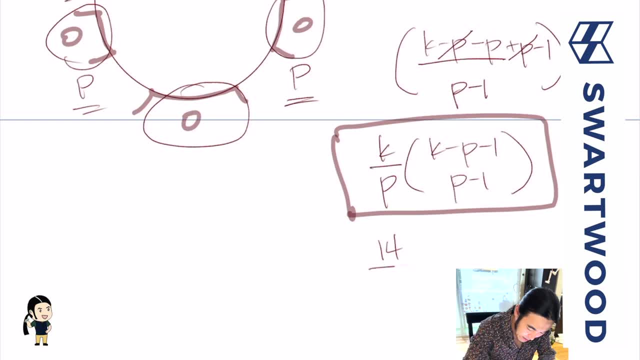 previous case we had. so. in our previous case, K was 14. the number of nights picked was 3. we had 14 minus 3 minus 1. choose 3 minus 1. that's exactly what we had before. okay, so, but we can make this even more general. so the final version: 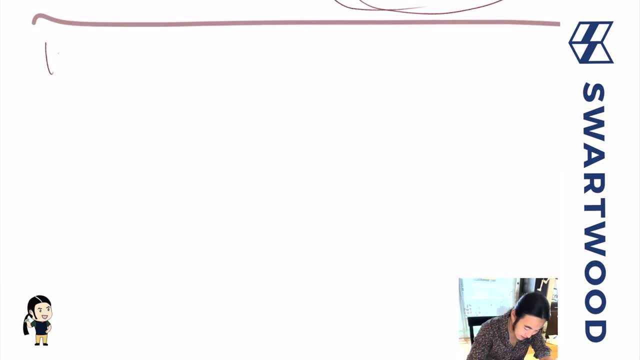 of this. let's have K nights, let's pick P of them, but now let's have s nights, at least s, so at least s nights in between each pick night. okay, that's my shorthand for it. so let's follow the same procedure and this might be even quicker. so we 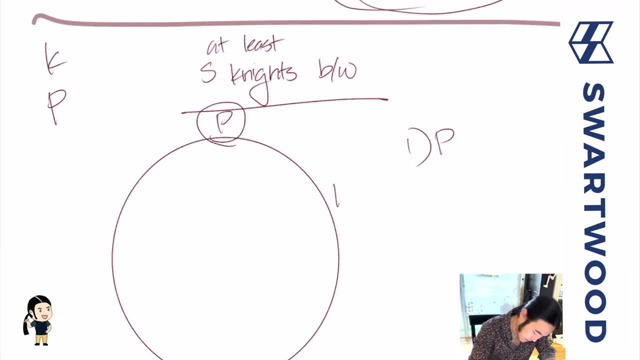 pick again Percival, place Percival here. then we imagine there's some other number of nights. it's gonna look identical to what we did before. okay, so we place all of them down. how many nights do we have? well, we have the K nights. we place Percival and the other pick nights we're gonna subtract all of. 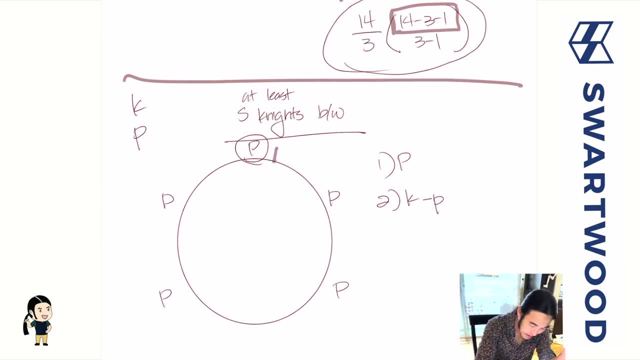 P Okay, But now the stipulation is we need to have at least some number of nights between each of these. So with P nights there are P gaps between them at the round table, And so I think again we need to put down at least one, two, three, dot, dot, dot P nights in between. That 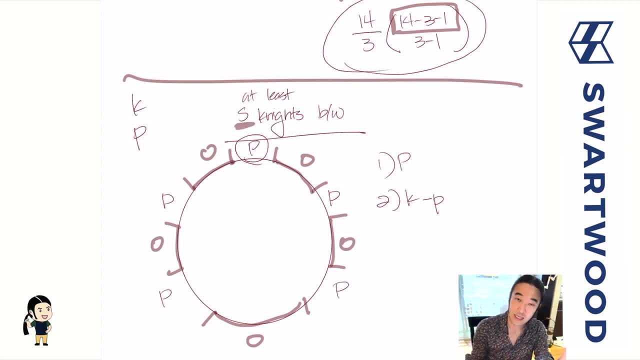 went before. Remember, between each night, we need at least S nights. So each of these isn't P, it's really S nights in here, S nights in there, all the way around. Okay, So total number of nights we actually need to put down is S P. Okay, I've said it's not that great, Let me make it. 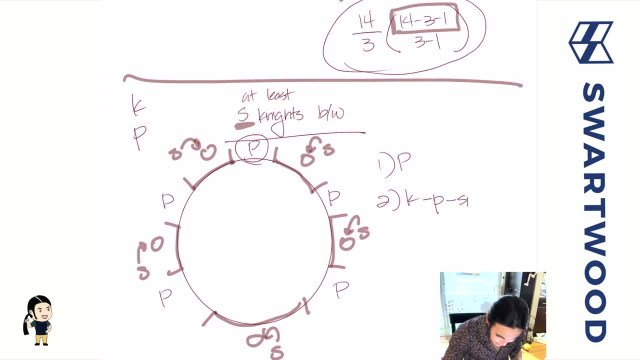 a little better. Okay Is S P Okay. So now we've seen this game before. We have this many nights to place down. How many buckets do we have Still the same number: one, two, three, four, up to P. 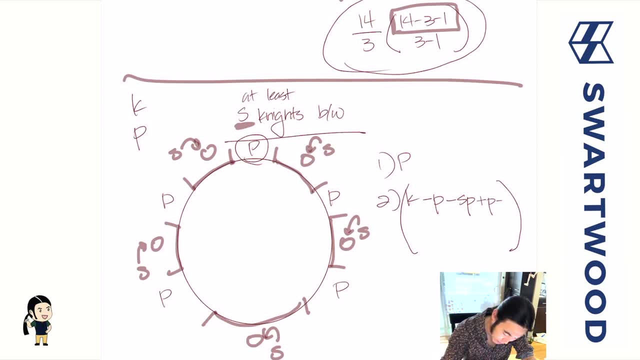 So it's going to be P buckets, which is really just P minus one. two, Choose where the P minus one guys go, the dividers. But just like before we started, Percival could have been any of the nights, So multiply by K, But then you have this sort of 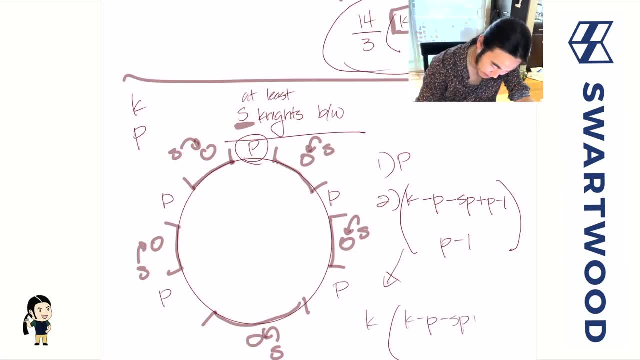 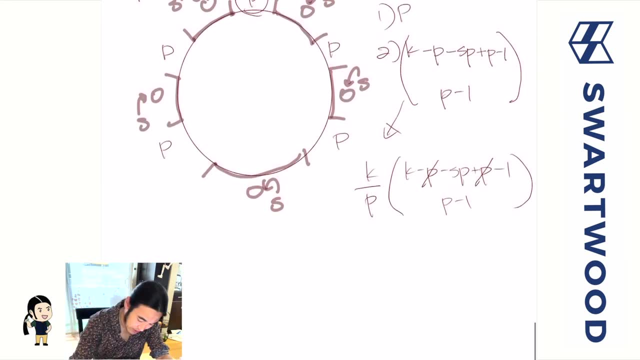 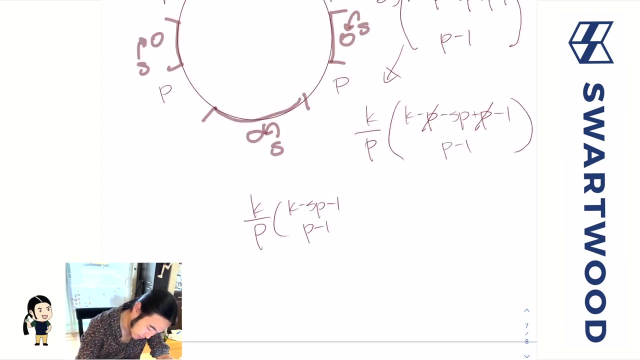 redundancy right, Because we distinguished one person one night, but really any night in the group is equivalent, So we need to divide by P. When we clean this up, we're going to get this And now we'll get K over P times, K minus S, P minus one, choose, P minus one, Okay. And if we go, 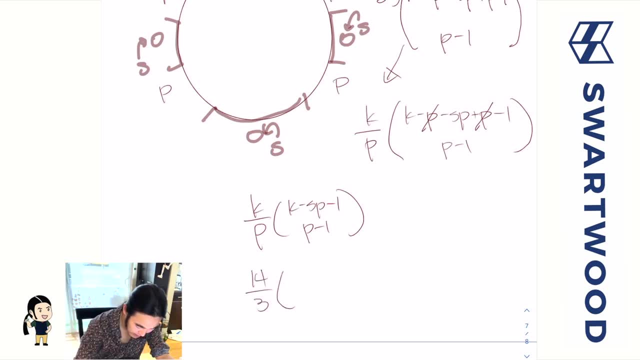 back and plug in the numbers from before. we'll get four, So that's going to be 14, three, 14 minus well, P was three, S was one. right, That's going to be three minus one. choose three minus one, And that's exactly the same answer as before. 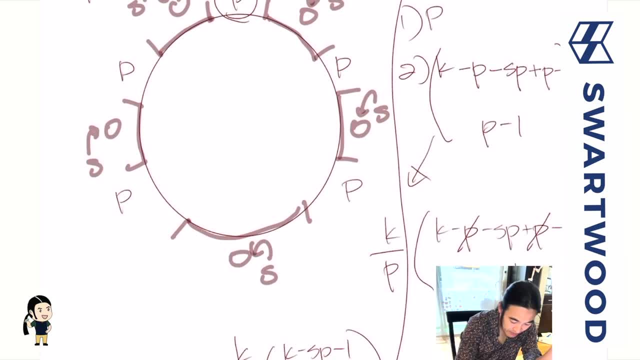 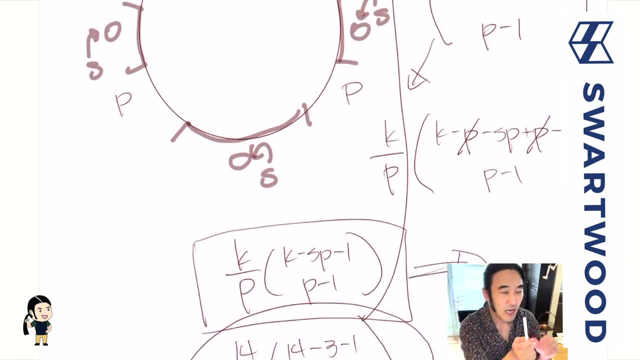 Oops, Okay, All right, No big deal. So this is very nice. The formula is actually really pretty And this is a classic problem. It's the most general case of this classic problem. Okay, I would ask you to check out the book that I mentioned before. It's actually by George Martin. 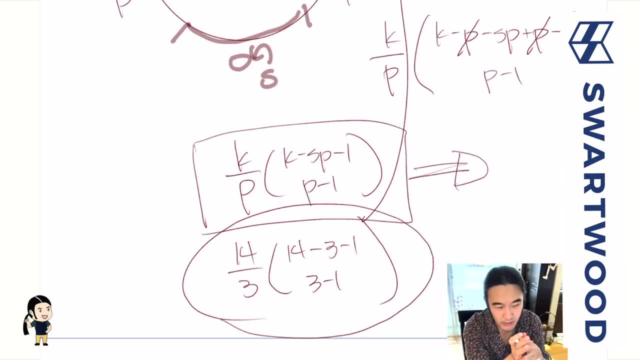 It's a great book. It does this differently. It does this differently. It does this differently And it does in a way where you're learning or practicing some new techniques. So obviously, if you want me to do that method, we can do that too. but hopefully this helped And I think after 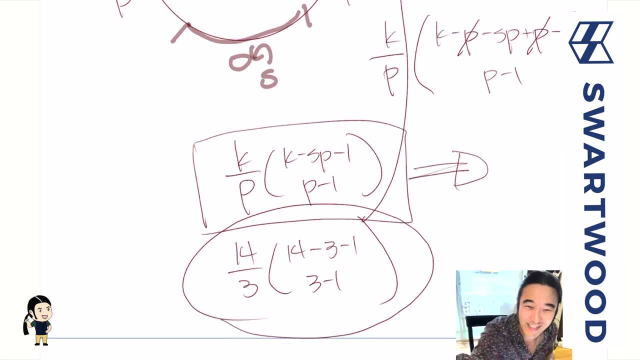 all these videos, you basically mastered the round table problem. Okay, I'll see you guys next time. 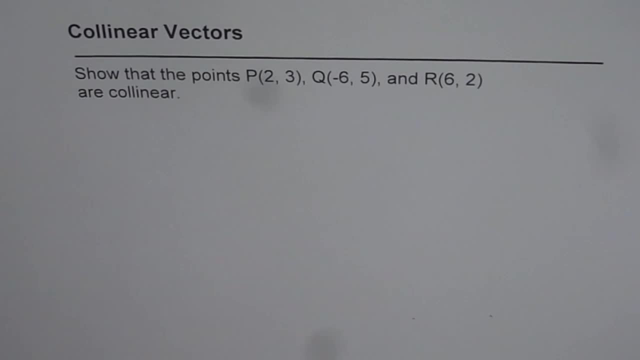 Collinear vectors Show that the points P, 2, 3,, Q minus 6, 5, and R 6, 2 are collinear. When we say that the points are collinear, that means that they lie on the same line. 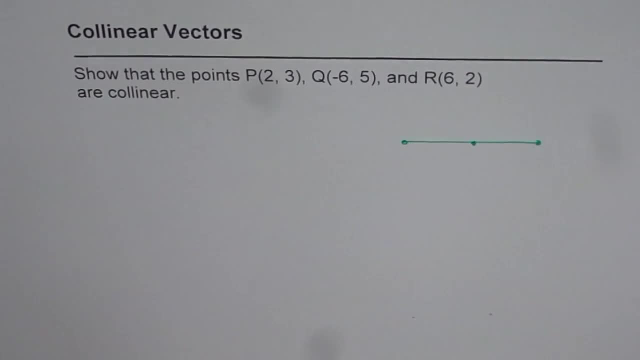 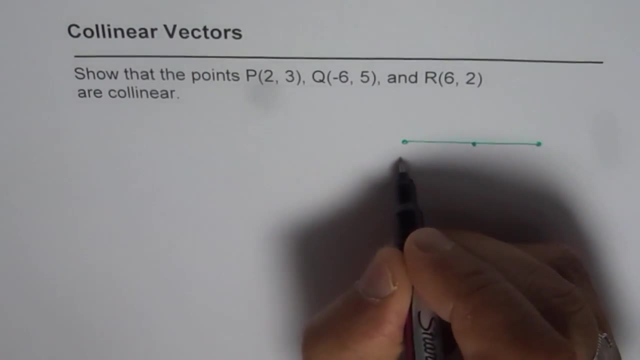 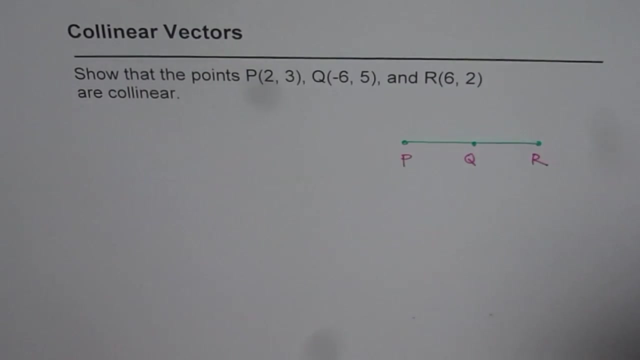 So that's what it means, right? So we are given three points and we have to just prove that they lie on the same line, So they are collinear. So what we need to prove here is, so, randomly, I'm just writing P, Q and R right Now. the points are 2, 3 for P, for 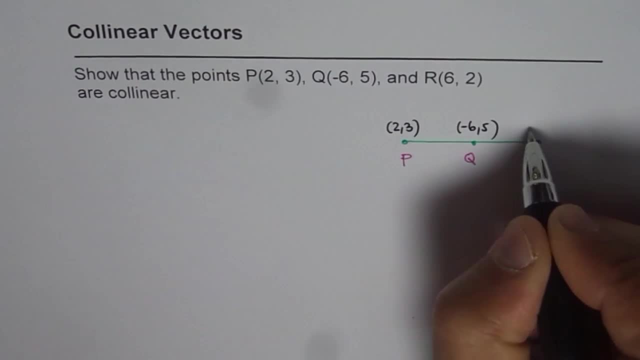 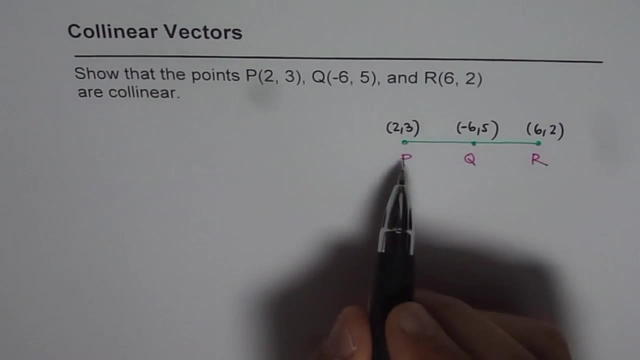 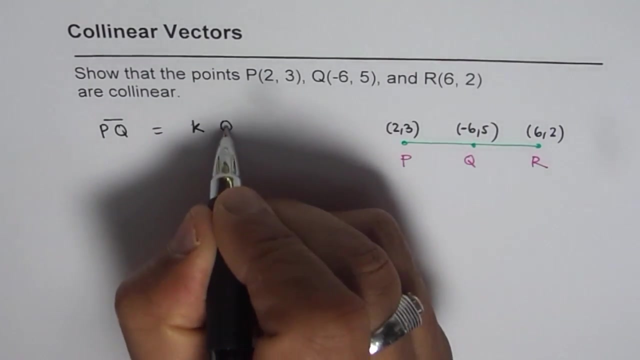 Q, it is minus 6 and 5, and for R it is 6 and 2.. So in case they are collinear, that means that P- Q should be equal to scalar multiple of Q- R. Then they are in the same line. 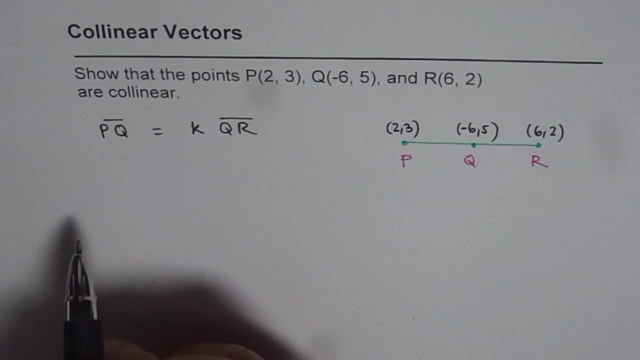 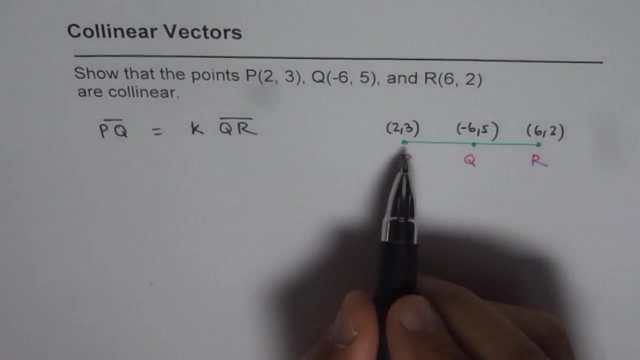 So let's find out the value of K. If we have a valid value of K, then they are collinear, Otherwise they are not. So from here, what is P Q? P Q will be equal to minus 6, minus.